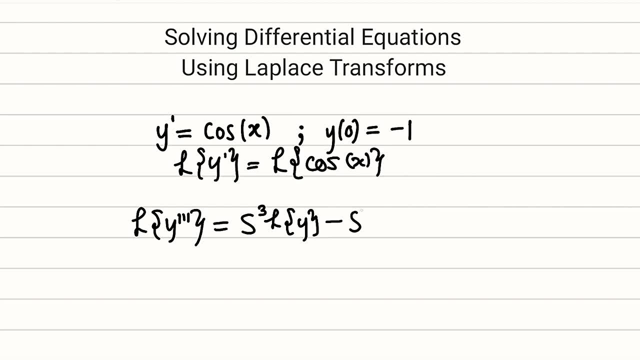 The power of s will reduce by 1.. We have s squared multiplied by y of 0.. You can see, we introduce y minus. the power of s will reduce by 1.. We have s squared multiplied by y of 0. Then, this time around, we have y prime of 0.. 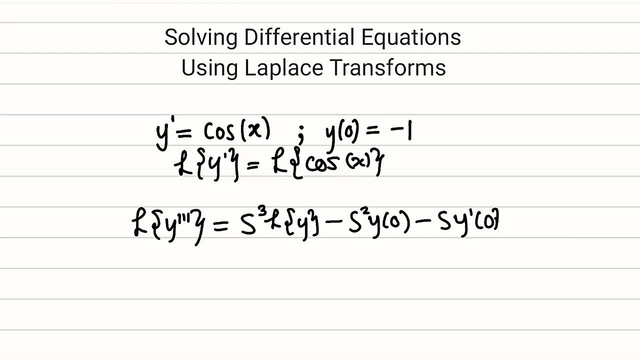 The order of our derivative is increasing, while the power of s is reducing. Then, lastly, you have to stop. when s vanish, The power of s will reduce by 1, so we have s power 0 equal to 1, but this time around we have y prime, prime of 0.. 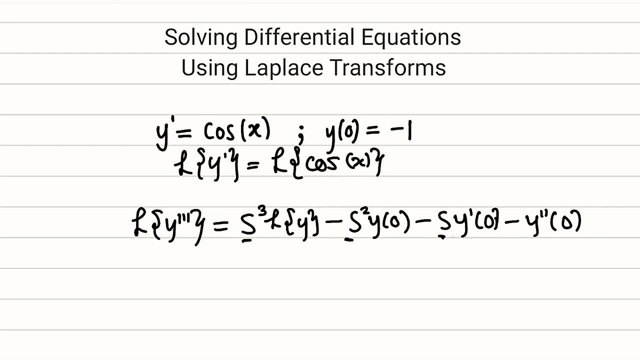 If you look at this pattern, the power of s is reducing, but the order of derivative is increasing. What if you want to find the Laplace transform of y, prime prime, which is double prime? This is equal to s squared, because the order is 2, multiplied by Laplace transform of y. 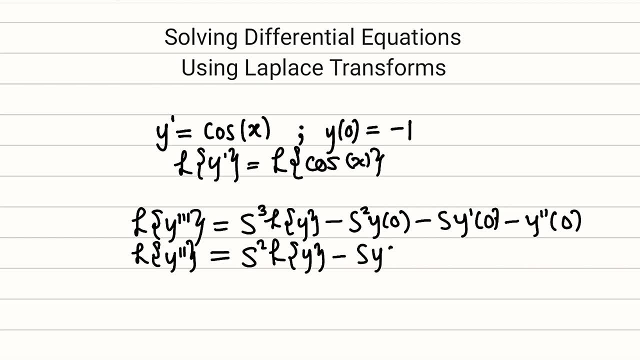 minus, the power of s will reduce. We have s y of 0. This time around s will vanish. in the third term We have just y prime of 0.. And if you want to take the Laplace transform of y by 1 to the power of s, what you need to do is we are going to subtract. 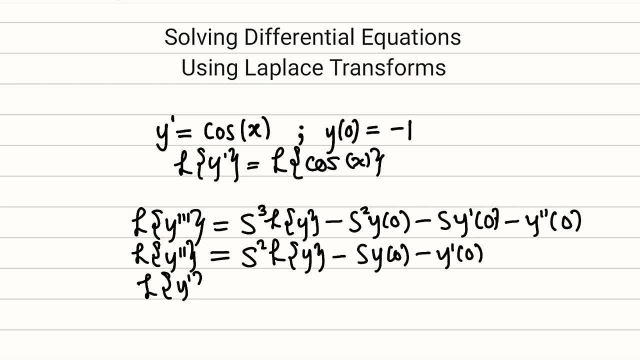 the laplace transform of only y prime. this is equal to s, because the order is one multiplied by the laplace transform of y. then minus s will vanish. we have only y of zero. all right, so now you can see that the laplace transform of y prime is equal to s multiplied by the laplace transform. 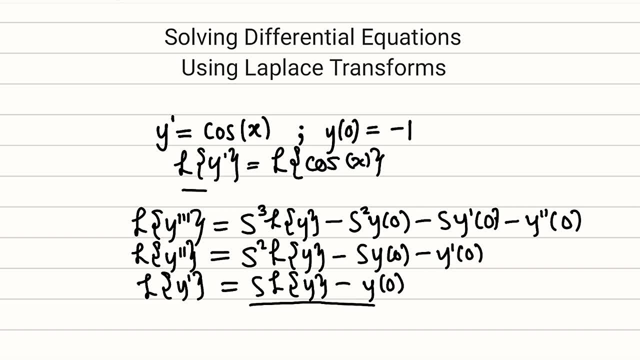 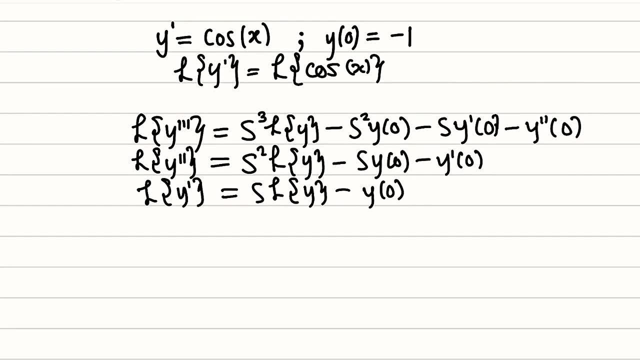 of y minus y of zero, which we have to substitute here to the left. so let's continue solving our problem. to the left, we have s multiplied by the laplace transform of y minus y of zero. this is what we have to the left. so what if we want to find the laplace transform of cosine x? 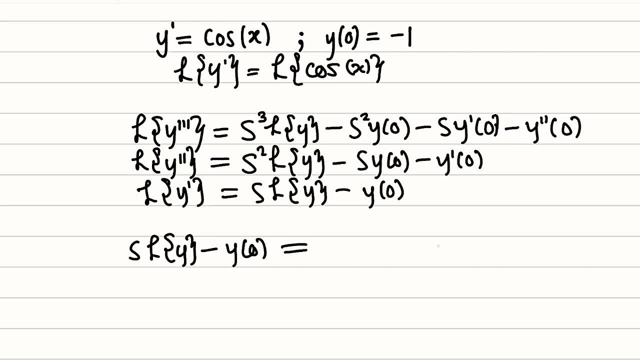 remember, in our introduction to laplace transform, we have learned that if you want to take the laplace transform of cosine of bt, this is equal to s divided by s squared plus b squared, where b is the coefficient of t. but this is a function of t. we are dealing with a function of x. therefore we can replace. 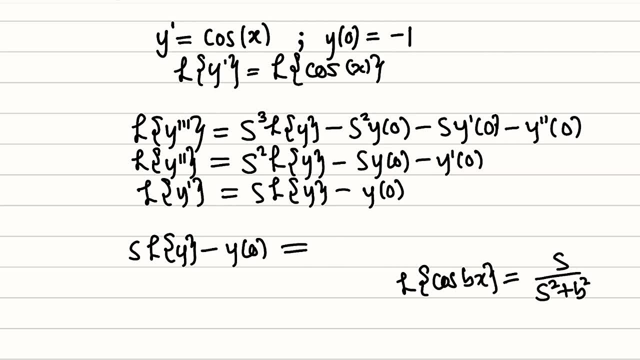 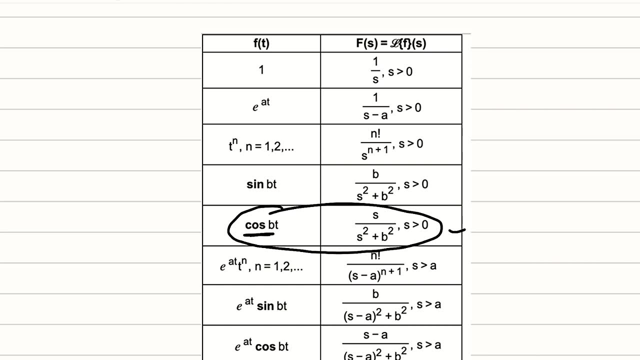 t with x. so we have x instead of t and the function remains the same. but let me show you this under a table. i don't want to be giving you everything of head. can you see that whenever you take the laplace transform of cosine bt, you end up with s divided by s squared plus b squared. 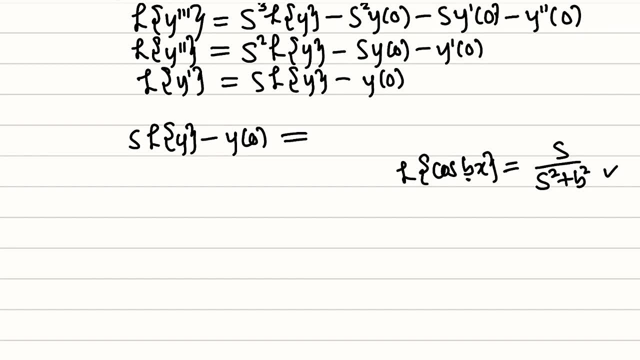 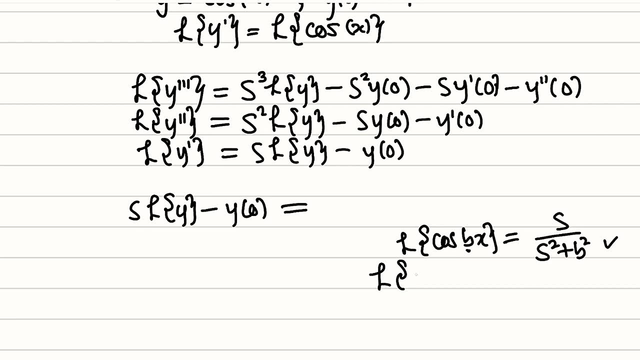 all right, but here our b is equal to one. from the right hand side, can you see that we have only cos x? therefore, the laplace transform of cosine one x- let me call it one x- will be equal to s divided by s squared plus one squared, because b is equal to one. 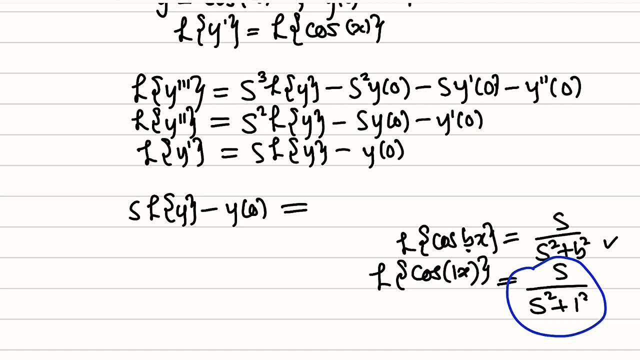 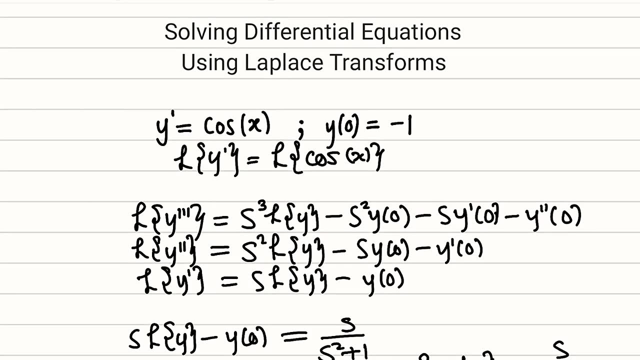 so this is what we need to substitute. to the right hand side, therefore, we say: this is equal to s divided by s squared plus 1 squared, which is the same thing as 1. so now let us substitute our initial condition. you can see it here: y of 0 is equal to negative 1. 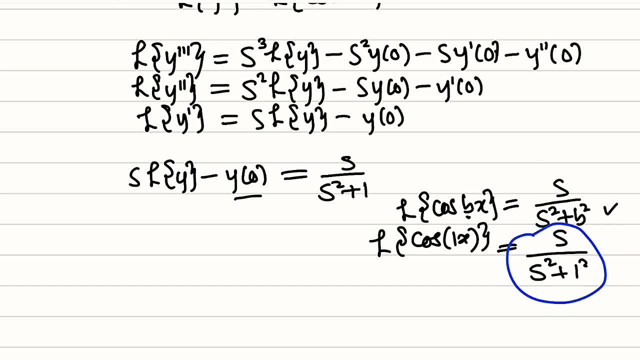 instead of y of 0 we write negative 1, s multiplied by the laplace transform of y minus minus 1. and to the right, we have s divided by s squared plus 1. the whole of this becomes 1, because minus minus is plus, so we have s multiplied by the laplace. 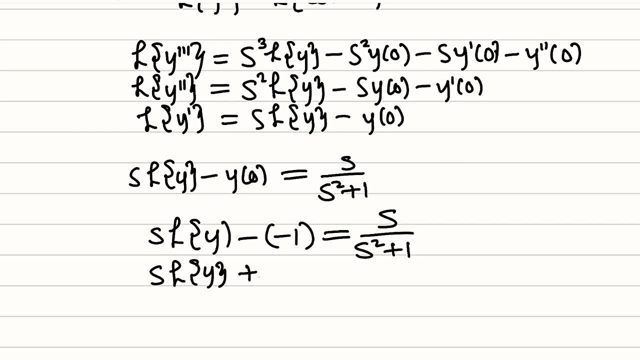 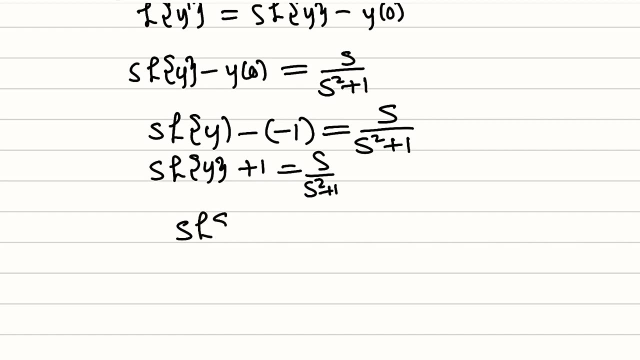 transform of y plus 1, and this is equal to s divided by s squared plus 1. now we are free to take this one to the right and it is going to become negative. we have, to the left, s multiplied by the laplace transform of y, and to the right, we have s divided by s squared plus 1. 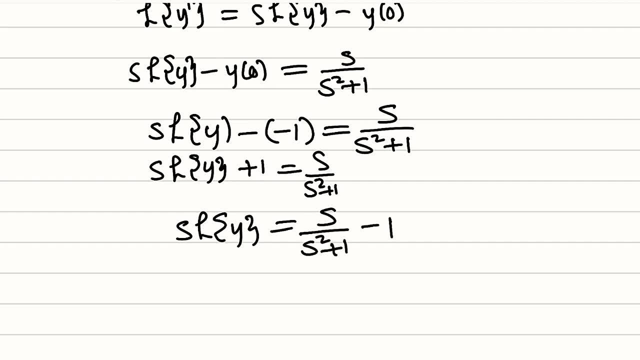 then minus 1, but this minus 1. we can rationalize it as 1 divided by 1 and if we like, we can multiply the top and the bottom by s squared plus 1 to have a common denominator. so this becomes s squared plus 1 divided by s squared plus 1. now we are free to simplify the numerator. 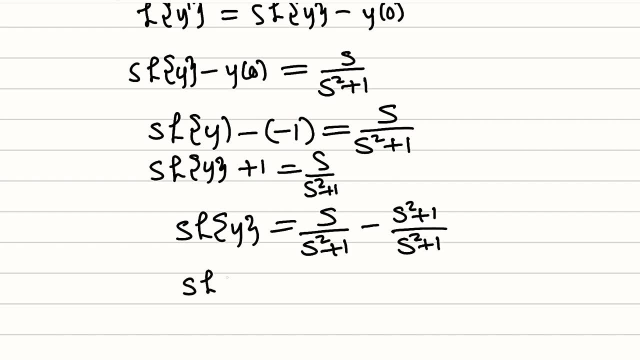 to the left, we have s multiplied by the laplace transform of y, and to the right, we have s multiplied by the laplace transform of y. this is equal to s minus s squared minus 1, because this minus will affect every term here. divide by the common denominator s squared plus 1. 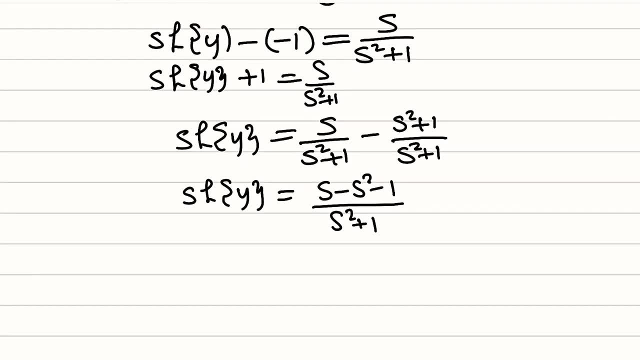 we need only laplace transform of y to the left so we can divide both sides by s. the laplace transform of y will now be equal to s minus s squared minus 1, divided by s multiplied by s squared plus 1. now you can see that the right hand side 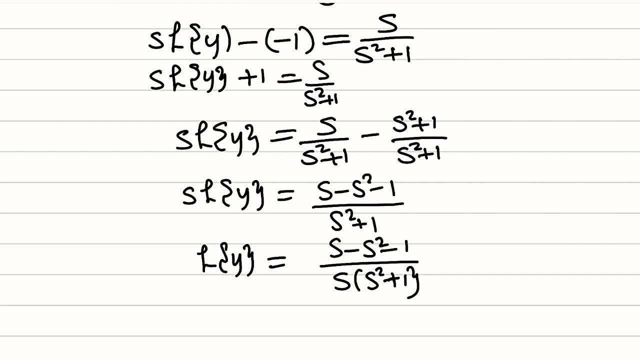 is just a compound fraction that we need to dissolve into a partial fraction, and this can be written as: a divided by s, which is the first factor, plus bs, plus c, byWell, if we solve these problem and not the left, still a perfect and place them at. 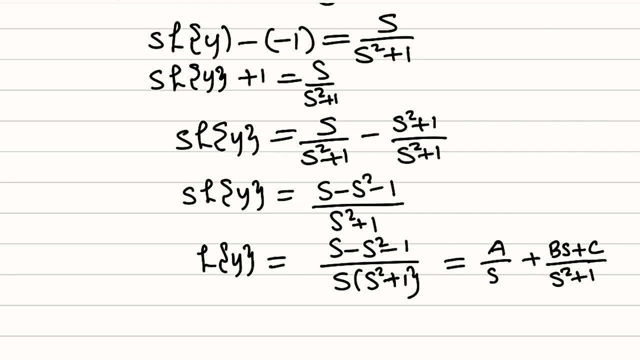 solving the problem. the right side should be positive. So lets see the answer for few more questions. why we have a constant here to the top is because the denominator is a linear function. therefore, the denominator will be a polynomial of 1 Ist, 0 den and 1 ist is just a constant. here we need to have a linear to the ي' is. 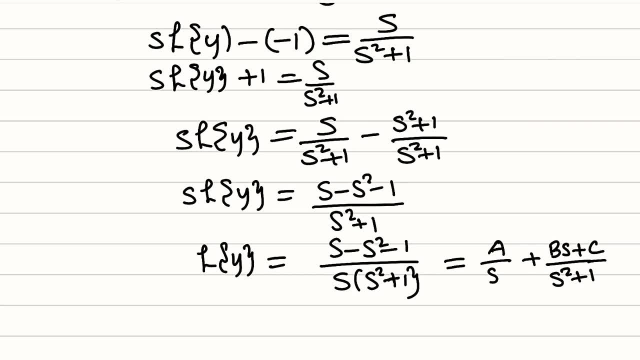 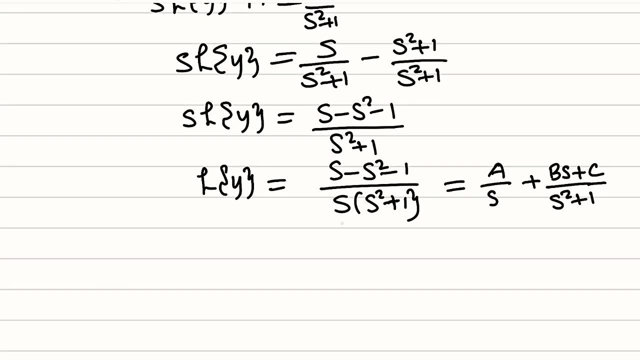 a difference if we construct here the bottom is quadratic and 1ist is a difference, because a bottom is quadratic and here we have to a linear to the top piece and t that gives the quadratic will be a linear polynomial. all right, so, um, let us clear the fractions by multiplying. 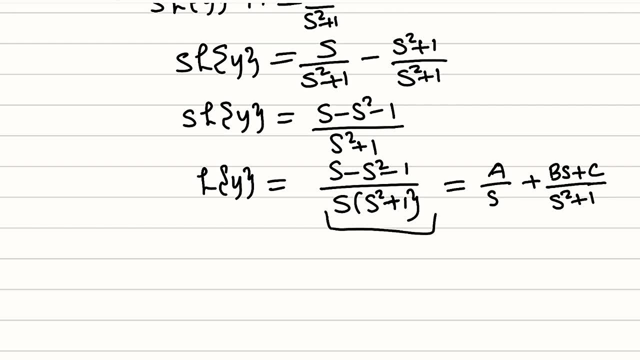 each term by s multiplied by s squared plus one. if you do that, to the left, you have only the numerator s minus s squared minus one, and to the right, take this. multiply by this s will cancel s, leaving only a, a multiplied by s squared plus one. do the same thing here. take this: 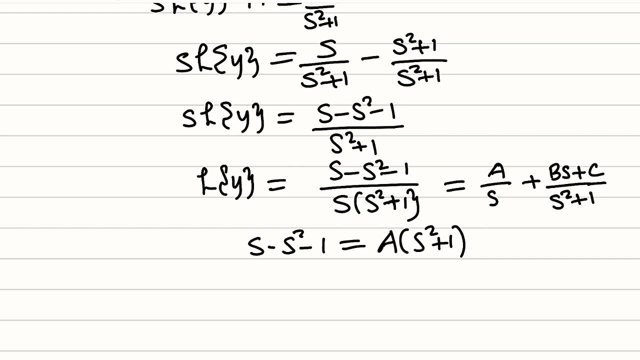 multiply by this s squared plus one will cancel s squared plus one, leaving s multiplied by b s plus c. now let us expand this parenthesis: s minus s squared minus one. this is equal to distribute a. inside the first parenthesis, we have a s squared plus a. do the same thing to the other. 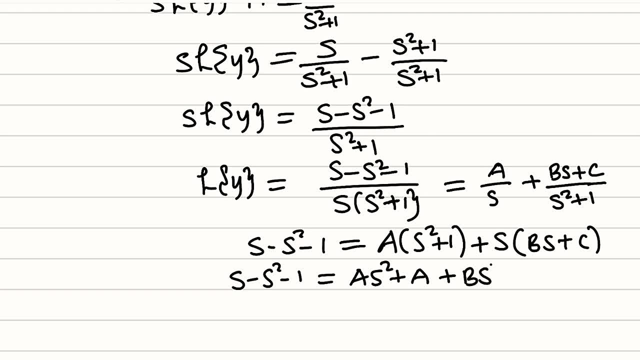 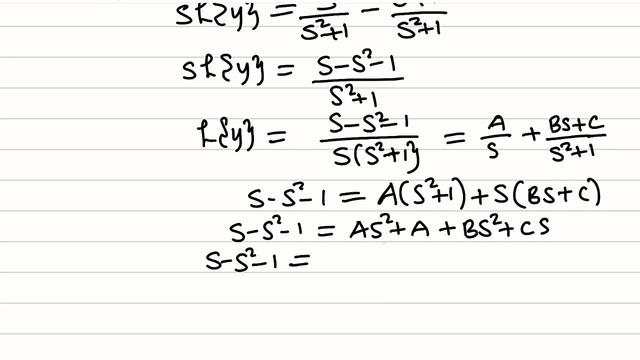 one s multiplied by b s, is b s squared, then plus c s. all right, let us bring those with s squared together: s minus s squared minus one, this is equal to. we have one here. we have the other one here. you can even factor out s squared, so we have a. 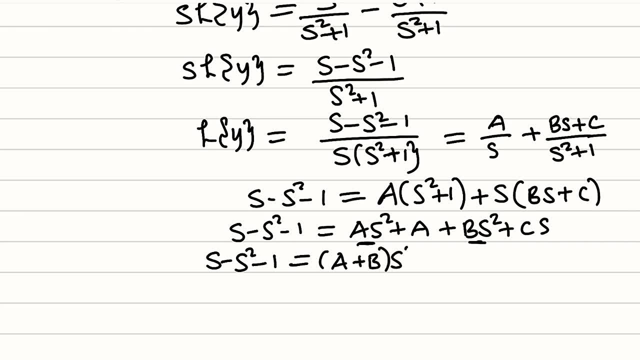 plus b, multiplied by s squared, then those with s, we have only c s, and the constant, we have a. okay, we are going to solve this equation by relating the coefficients. the coefficient of s squared to the right is a plus b, and the coefficient of s squared to the left is negative one. you can see. 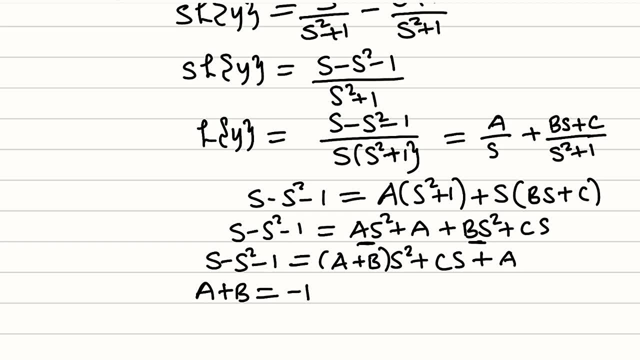 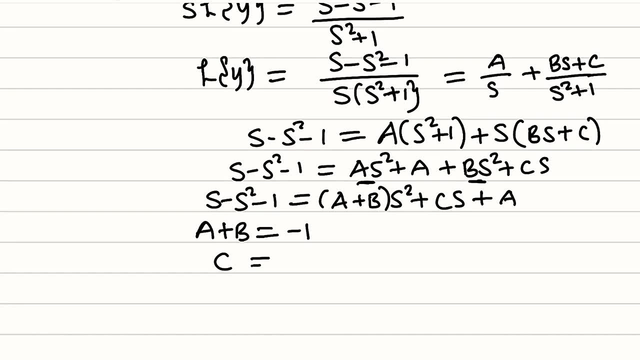 it here, so this becomes negative one. take the other one: coefficient of s to the right is c and the coefficient of s to the left is a one. the constant a will be equal to the constant to the left. negative one. now you can take this value of a, which is negative 1, plug it back into the first equation to get the value of b. 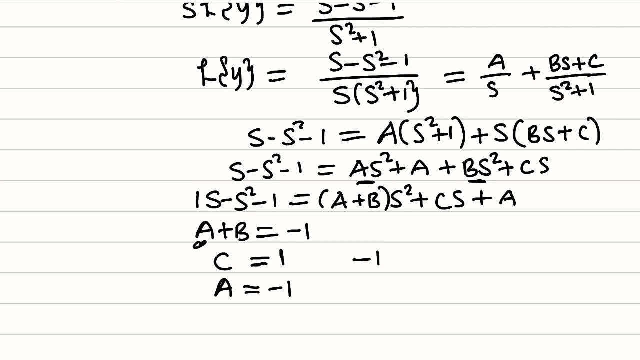 okay, so we have negative 1 as the value of a plus b equals negative 19 p at 18, three, where negative 2 equals no, that would be equal to b2 plus 1. so we have negative 1 as the value of a plus b. 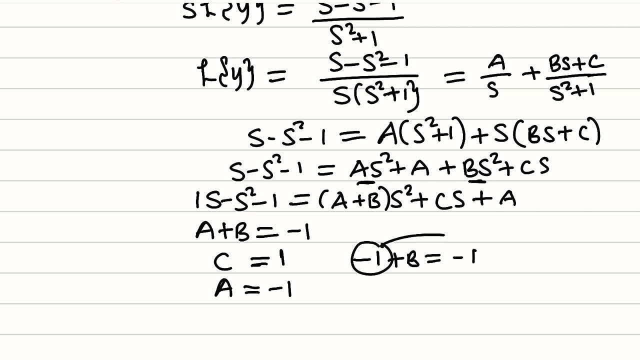 here. you can remember when I told you that you can use it if you just work with it in one way that does not General Graphs. so multiple может ke X. you should know this. negative 1.. Take this to the right. it becomes positive and positive. 1 plus negative 1 is 0. so 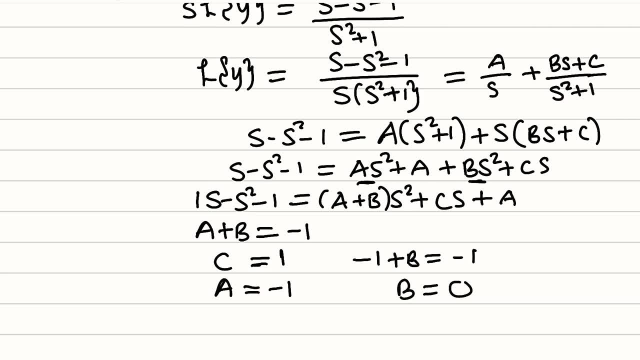 b equals 0.. Now we have the values of a negative 1, b 0 and c equal to 1.. We are going to substitute them back into this partial fraction to obtain our required fraction. So let me copy that: Remember that this is the Laplace transform of y. 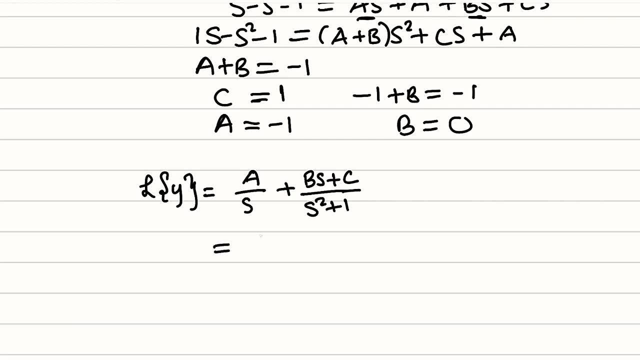 and this becomes: a is negative 1, so we have negative 1. divided by s plus b is 0. So the whole of this becomes 0. We only have c to the top and c is 1.. You can see it here. 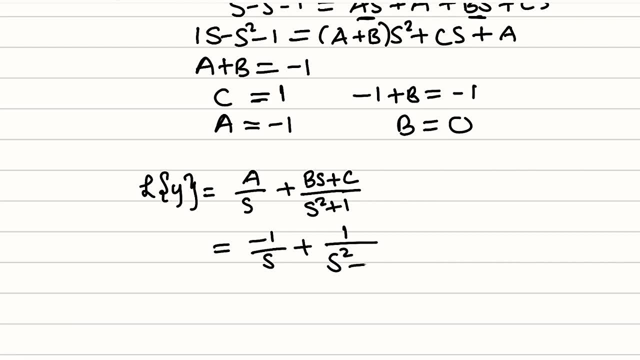 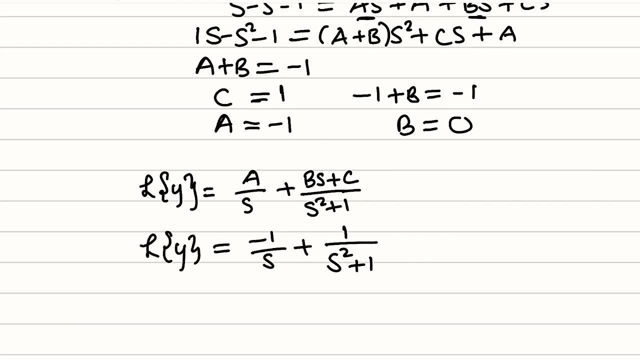 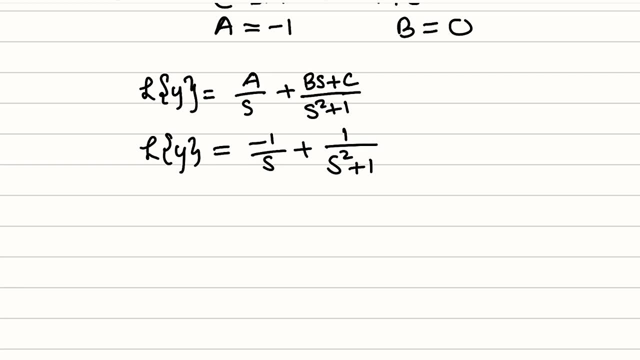 Laplace transform of both sides, Because we are looking for y. if you take the inverse Laplace transform of this, the inverse Laplace will cancel the Laplace, leaving only y, So y is equal to. you can take the inverse Laplace transform of these times independently, separately. 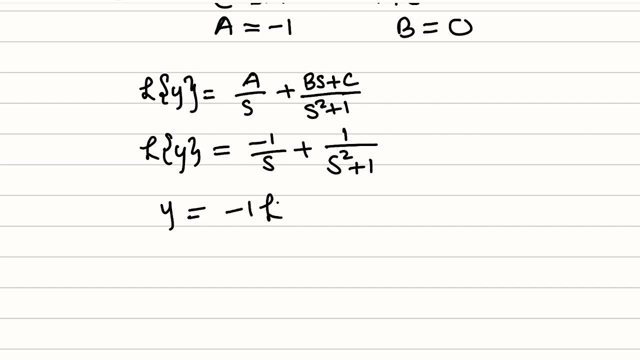 So we factor out negative 1.. We take the inverse Laplace transform of 1 divided by s, plus the inverse Laplace transform of 1 divided by s squared plus 1.. All right, So now let us go through our table to find the inverse Laplace transform of these two functions. The first one 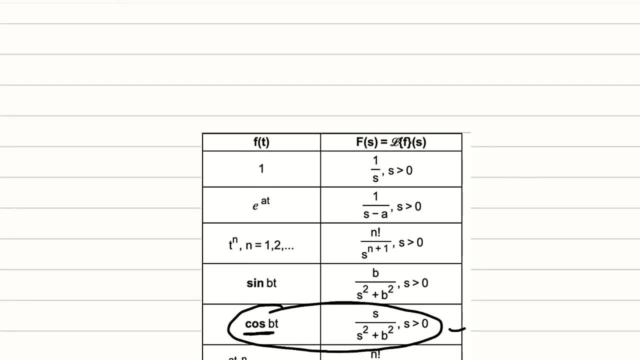 is 1 divided by s. Can you see that If you take the Laplace transform of 1, you're going to get 1 divided by s. Therefore, taking the inverse Laplace transform of 1, you're going to get 1. 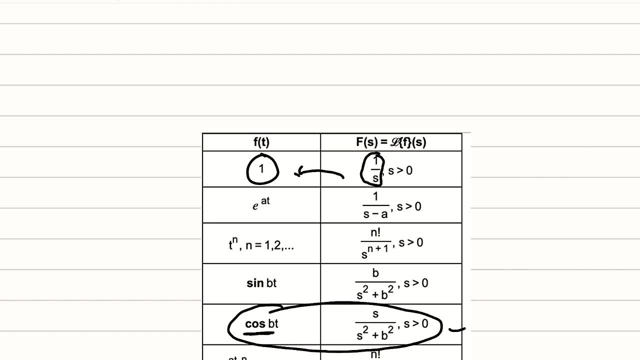 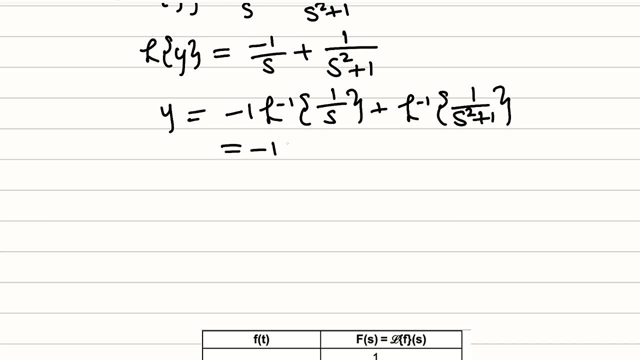 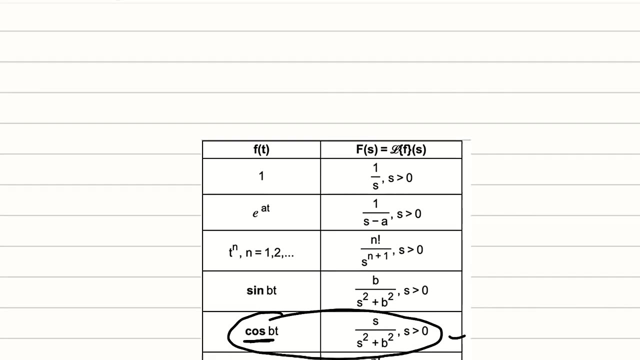 divided by s. Therefore, taking the inverse Laplace transform of 1 divided by s will give you back your 1.. Therefore, what we have there is nothing but 1.. This is equal to negative 1 multiplied by 1 plus. Now let us find 1 divided by s squared plus 1.. If you take the Laplace, 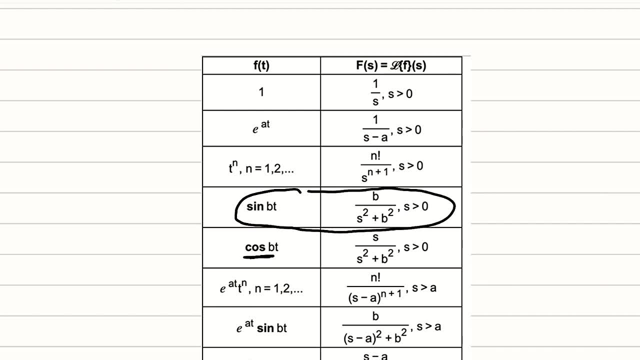 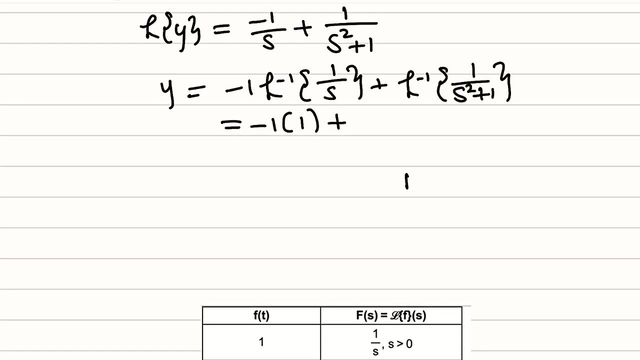 transform of sine bt, you're going to get b divided by s squared plus b squared. Therefore, if you take the inverse Laplace transform of this, you shall get this back. And now we are going to apply that here. Let me even write it here: The Laplace transform of 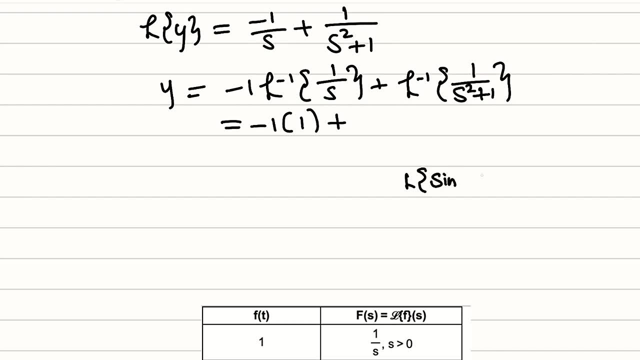 sine of bt is equal to 1 divided by s squared plus b squared. The same thing if you have a function of x Laplace transform of sine of bx. This will give us 1 divided by s squared plus b squared. What if b is equal to 1?? We have Laplace transform of sine. x will be equal to 1 divided by s squared. 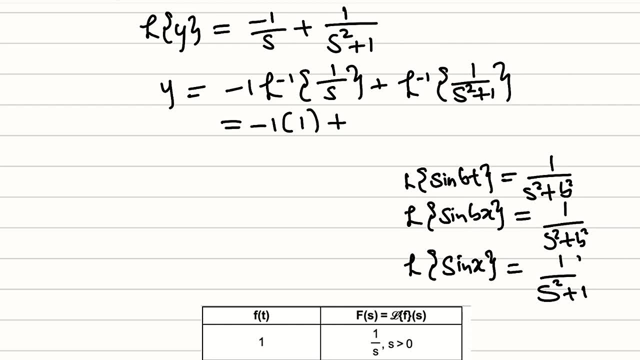 plus 1 squared, which is 1.. Can you relate? This is exactly equal to this. Therefore, if you take the inverse Laplace transform of both sides, this will give you back 1 divided by sine x. The whole of this is equal to sine x. Therefore, we write sine of x here. 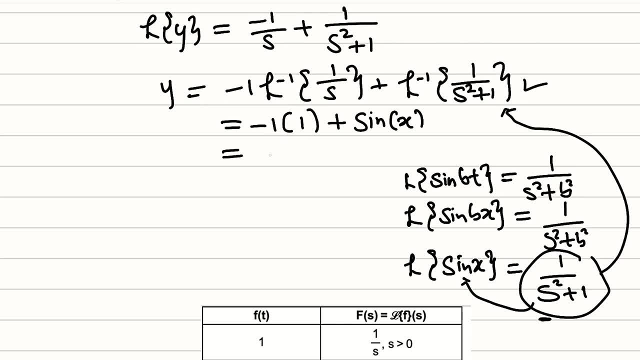 Negative 1 times 1 is negative 1.. So this finally equals sine x minus 1.. Therefore y, which is a function of x, is equal to sine x minus 1.. Wow, So now let us check by integrating both sides to see whether 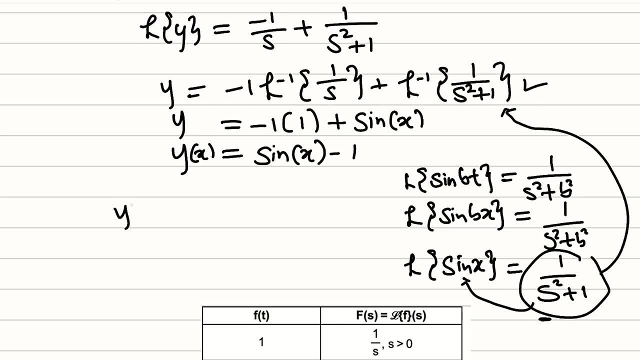 we are going to have the same function. Remember what we are having. initially is y prime equal to cosine x. If you integrate this with respect to x, you are going to get y. If you integrate this with respect to x, you are going to get sine x, plus constant of integration. 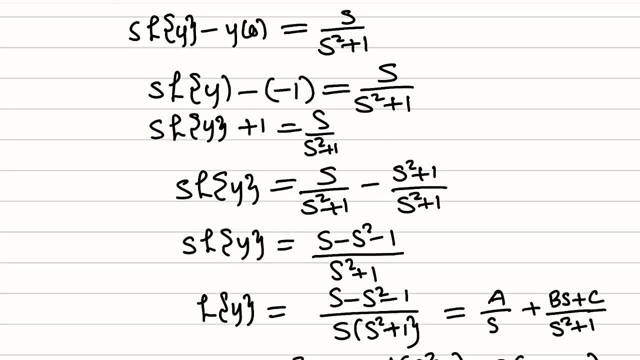 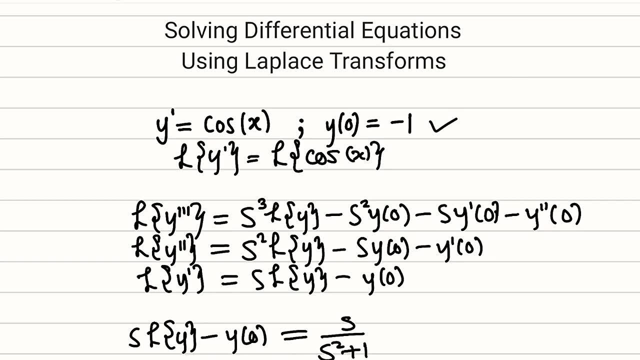 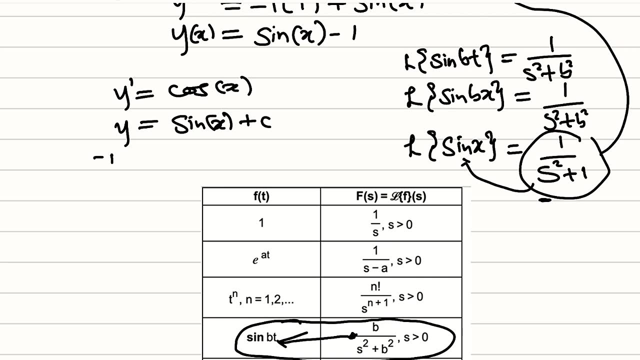 But remember, the initial condition says y of 0 is equal to negative 1.. Can you see that here? So we are going to substitute the value of x equal to 0 and y equal to negative 1.. This is negative 1 sine 0. 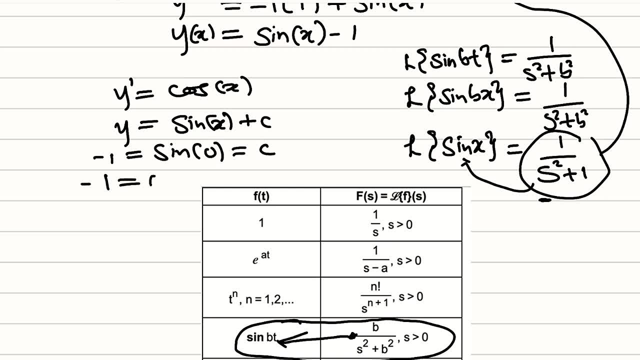 equal to c. Negative 1 is equal to 0 plus c. Therefore, c is equal to negative 1.. Sine of 0 is 0. Therefore, our solution becomes: we just need to substitute the value of c in this equation.